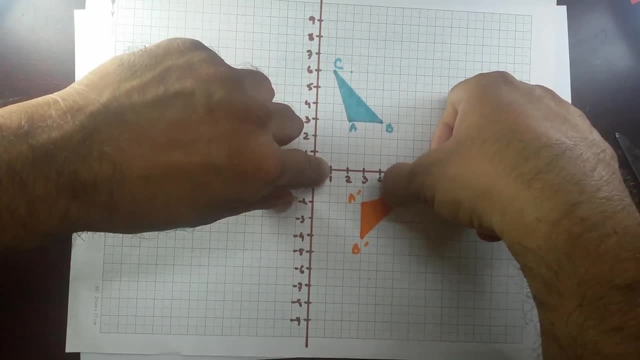 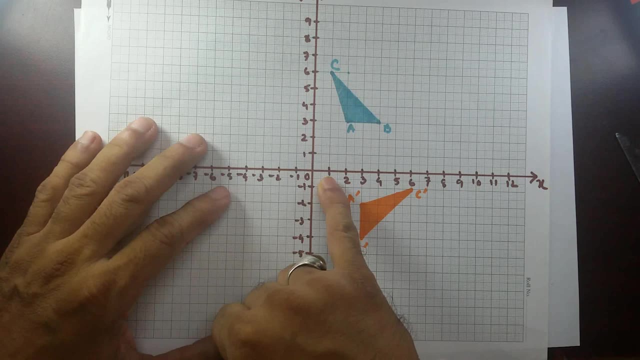 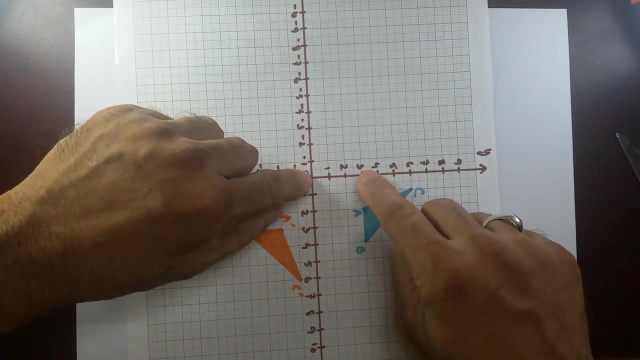 to the right and one unit below. So a prime is not over here. A prime is over here. So my prediction to the center to be 10. that was wrong. What about zero, zero? If I take zero, zero, then rotate this one. 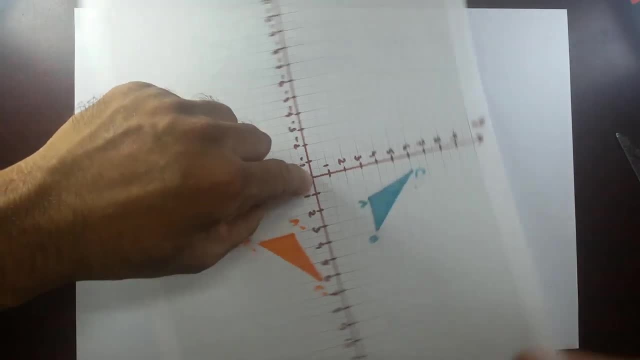 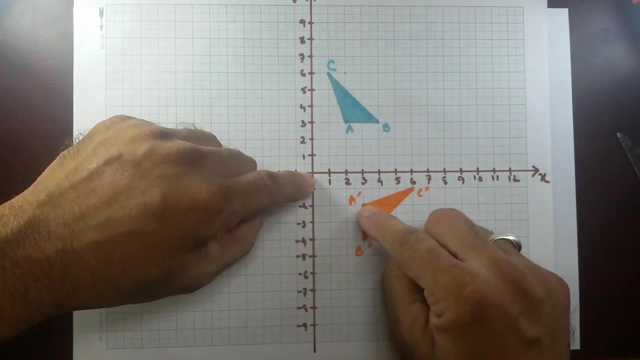 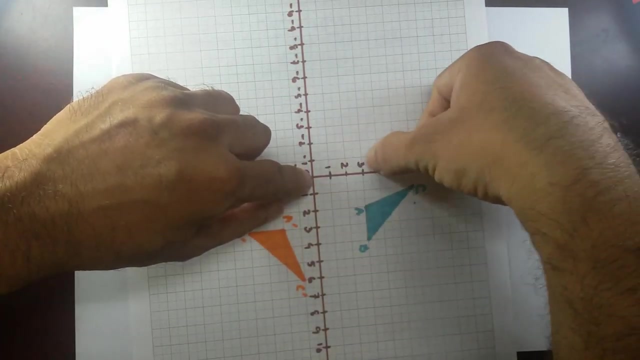 units to the right and two units below. so go back again. one, two, three to the right and two below. so this a comes to b, b, prime, a prime. let's try another one, see if, if, if this is correct or not, for c: one, two, three, four, five, six, six units to the right, one below. go back. one, two, three, four. 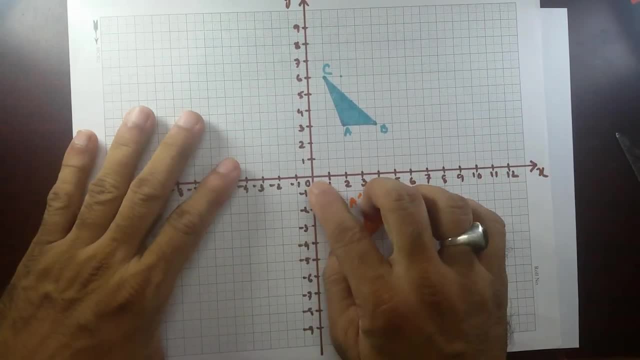 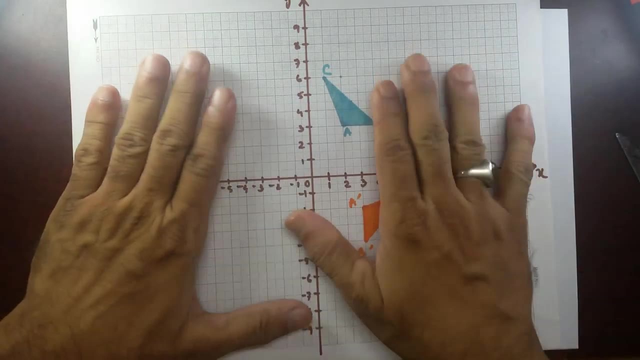 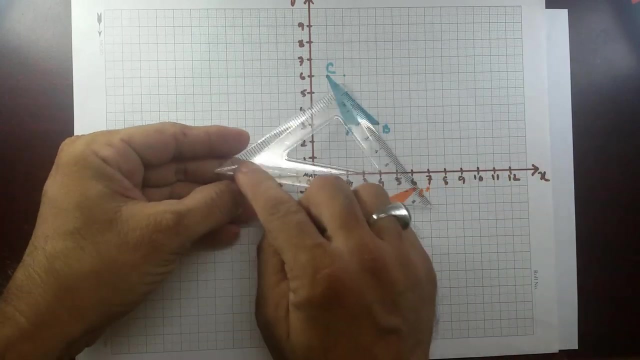 five, six and one below. so we are okay. now my prediction is zero, zero center, and direction is 90 degree clockwise. okay, now, this is one way of doing this. another way is if you are using the set square, okay, i'm using 45, 45, 90 degree set square. now this two corresponding point, any any? 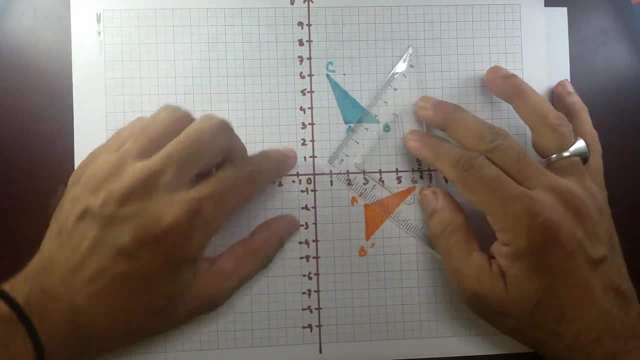 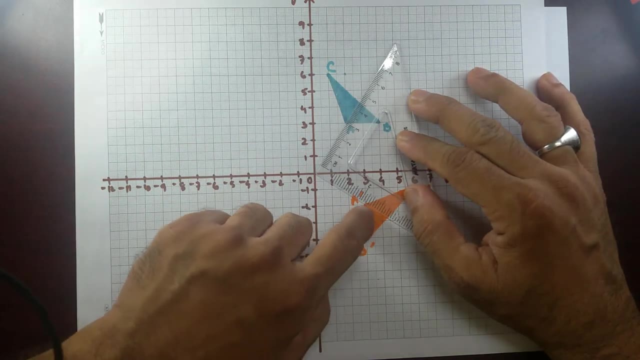 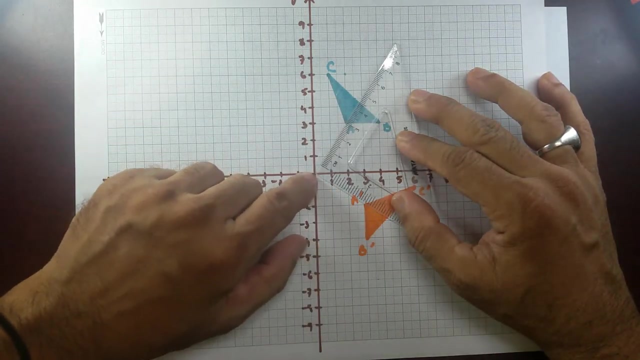 corresponding point will do one pair of corresponding point. okay, have this right angle in between them in a way, so that you can join, uh, this a and a prime, in a way. so this right angle comes to a point. okay, this point also shows zero, zero. okay, so this is: if you just join, that, 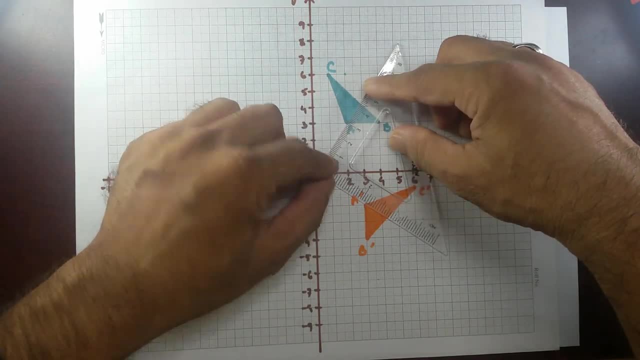 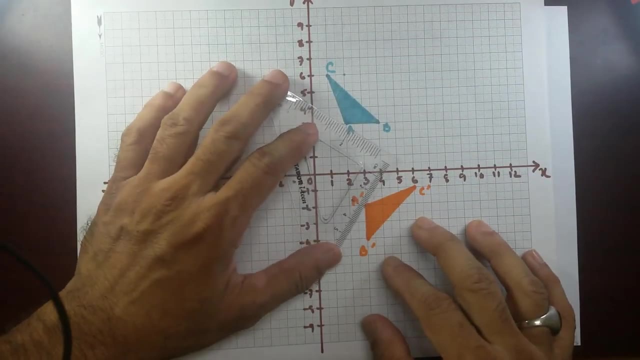 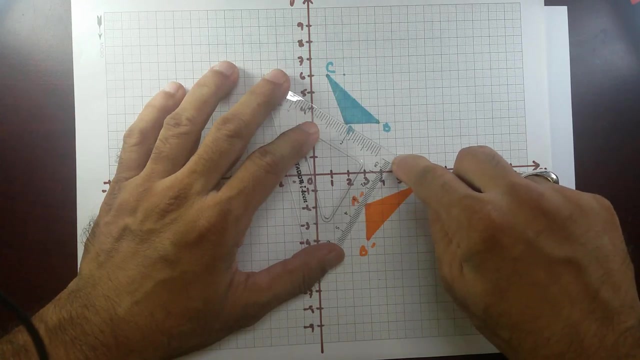 to corresponding point with the center. you can see that it's 90 degree and it's rotate this way: 90 degree, clockwise rotation. what if i do this way? of course i could do this way, okay, but when i do this way, the point showing somewhere, five one, the center, five one if the center is. 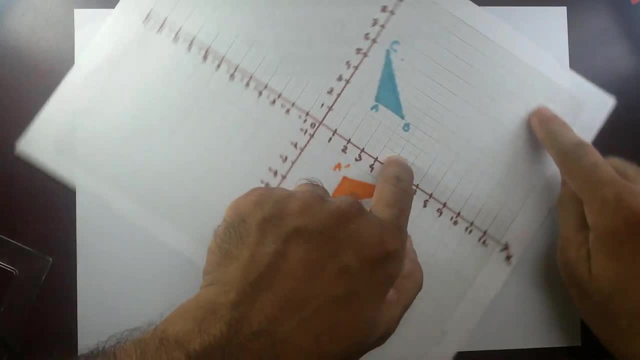 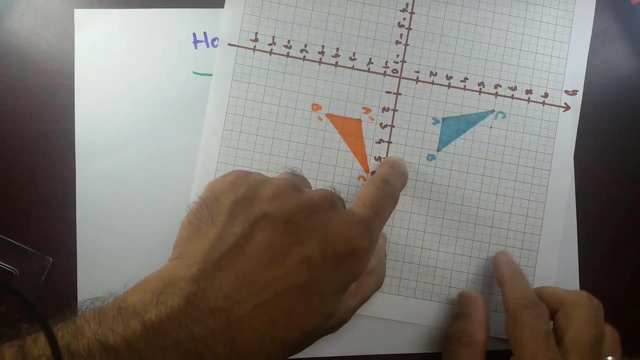 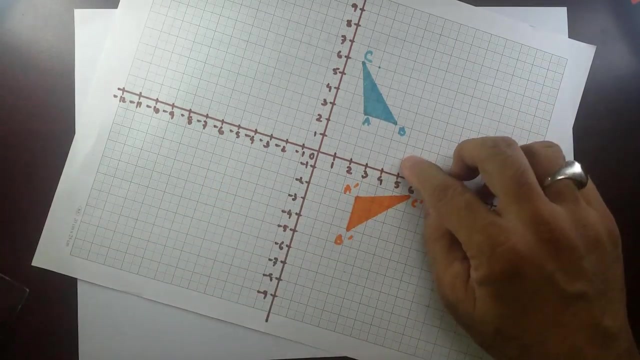 five, one. if we go like that, okay, 90 degree clockwise, see, my a would be one, two, two to the right and one, two, three up above. so go back: two to the right, one, two, three up above. there is no a prime, so this side is not gonna be the center of rotation. this side would be okay. so zero, zero. 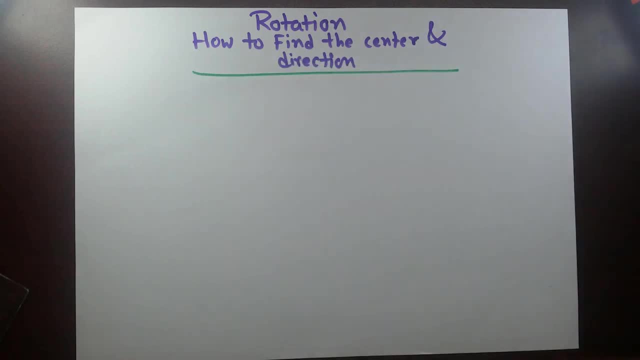 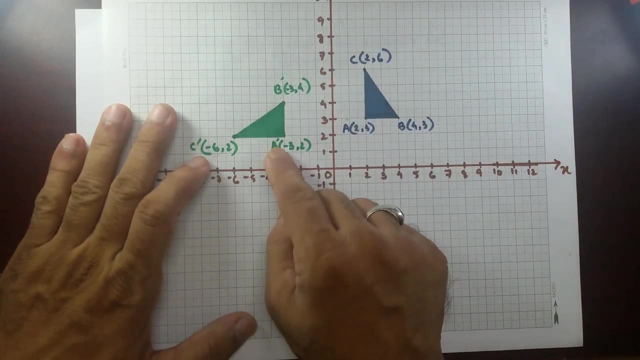 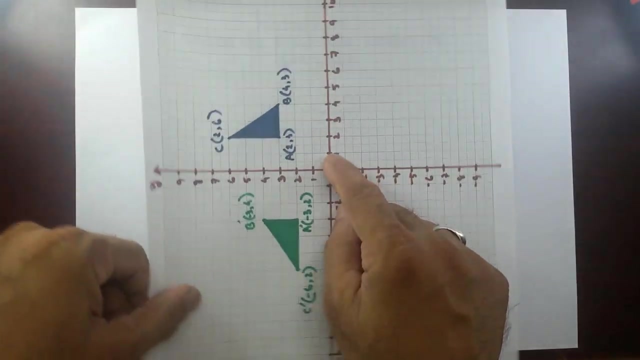 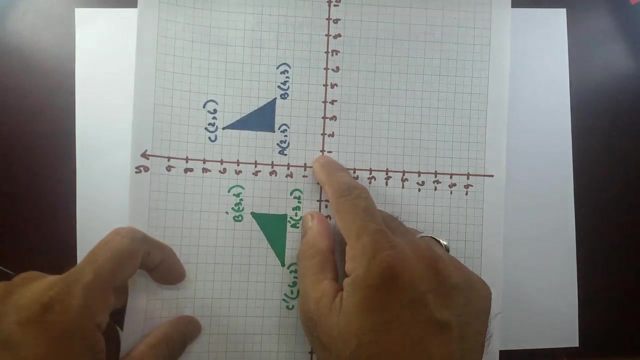 my center of rotation, all right, and same way if i'm using this one and uh a, b, c- this is the object again, and this side and the second quadrant, my uh image over here, and it seems like if i turn it this way then i'm gonna have this uh image. so this is 90 degree anti-clockwise and we're gonna. 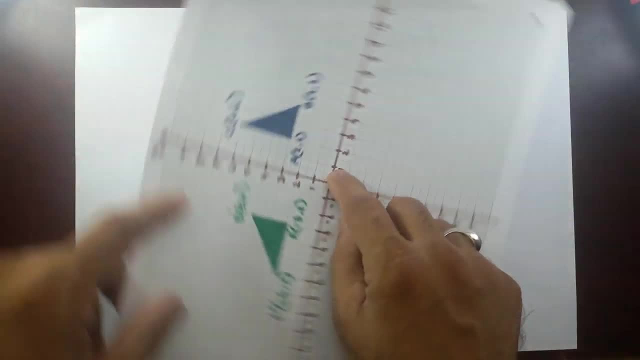 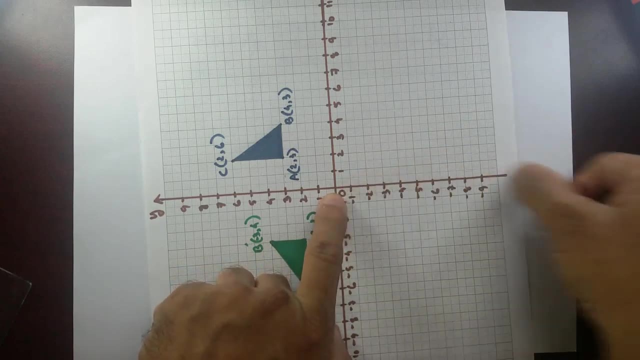 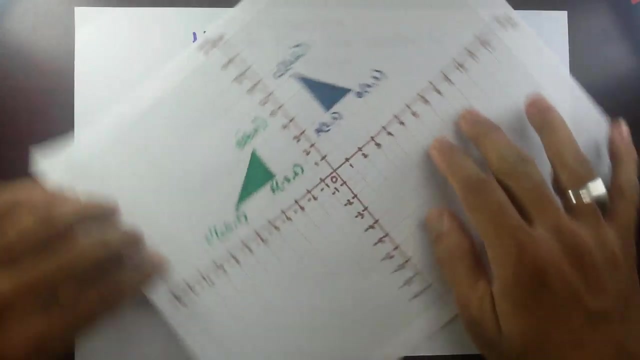 check it the same way. uh, when i, when i turn it around 90 degree, clockwise, anti-clockwise, this way, then this a comes over here. uh, now this is my x-axis: one, two, three, three units on the left of the x-axis and two units up. going back again to the original position: one, two, three, three. 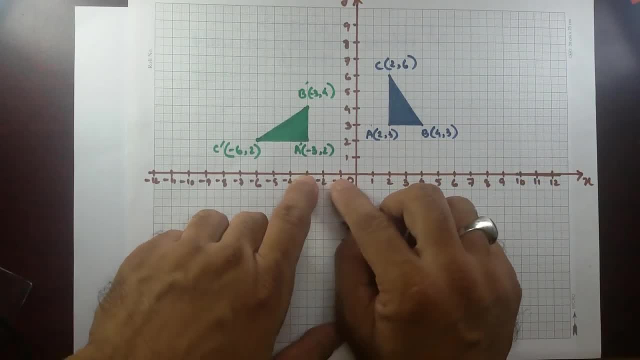 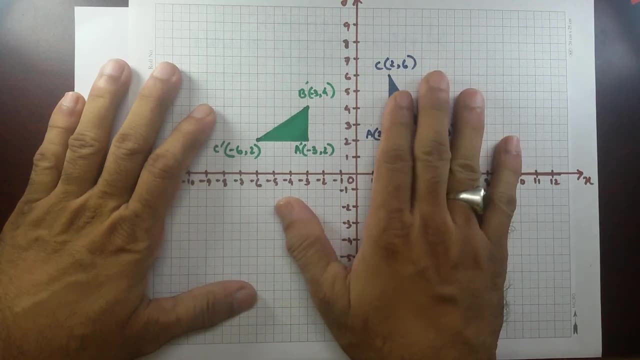 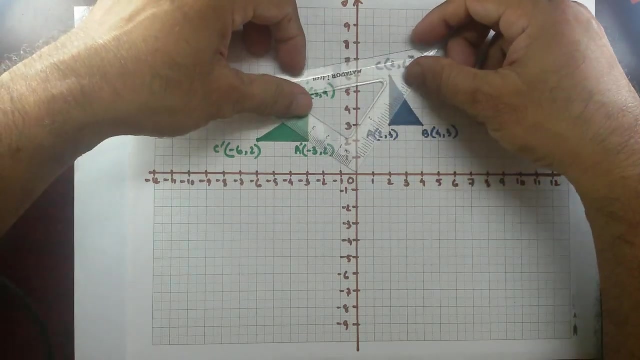 units to the left of this x-axis from the origin and then two up, so a a prime is okay. so this is my 90 degree anti-clockwise rotation. this is another way of doing this, right, okay, and remember the. the set is squared. we can use this and we can find out that it's 90 degree. okay, so. 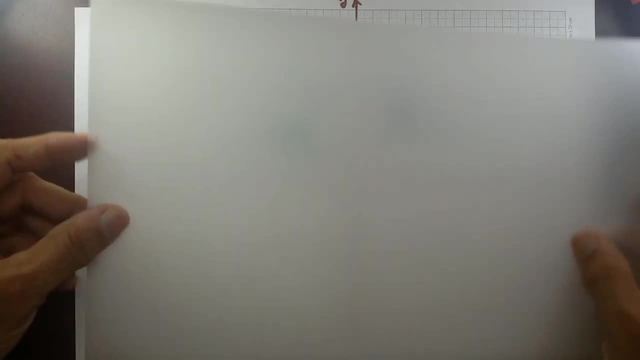 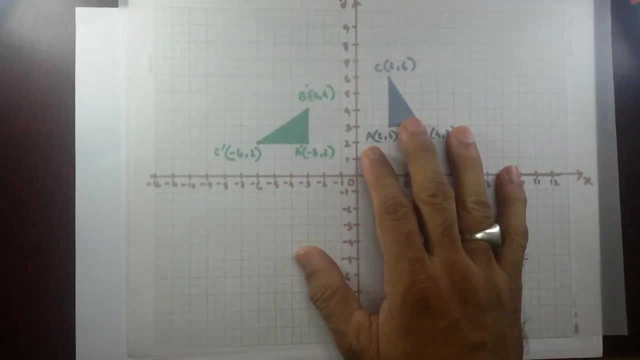 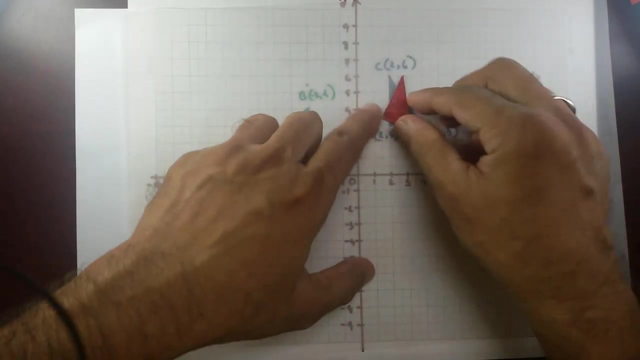 there is another, uh, interesting thing: tracing paper. we can use tracing paper to see the rotation. uh, we usually don't do it this way. all right, but we can. we can do this, we can do this. i'll just show you, even though i don't recommend it. nobody actually use it this way and i i don't think a lot. 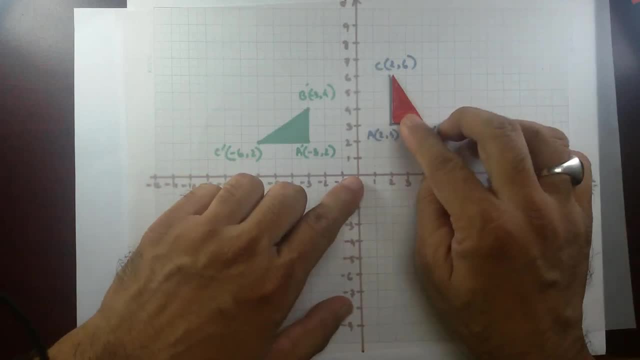 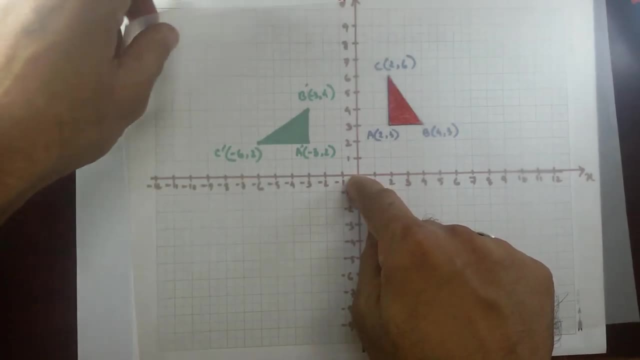 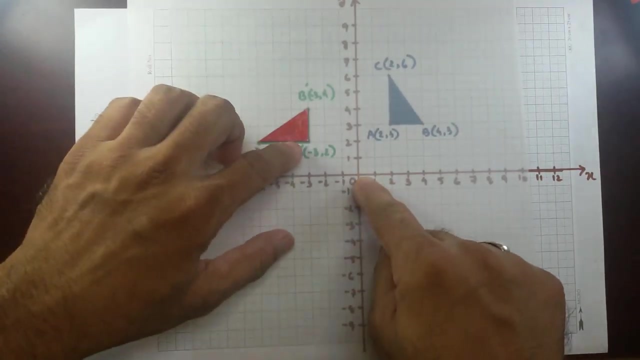 of student knows what tracing paper is. if my object is this one, and i put it over here and then my prediction, the center would be this: and i turn it around: 90 degree, anti-clockwise, see that it comes to that that place over here. so this is my image and center would be this: look at this, i'm 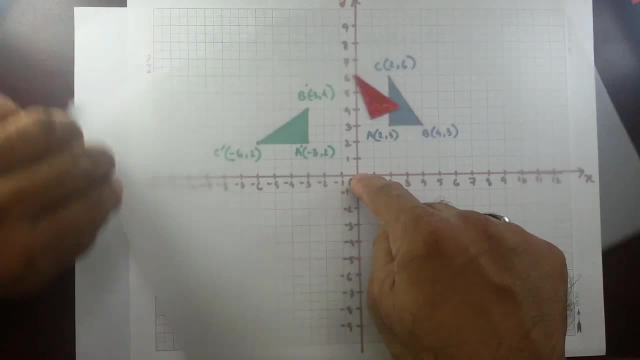 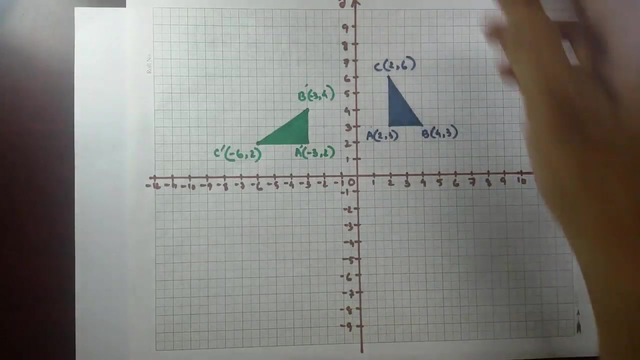 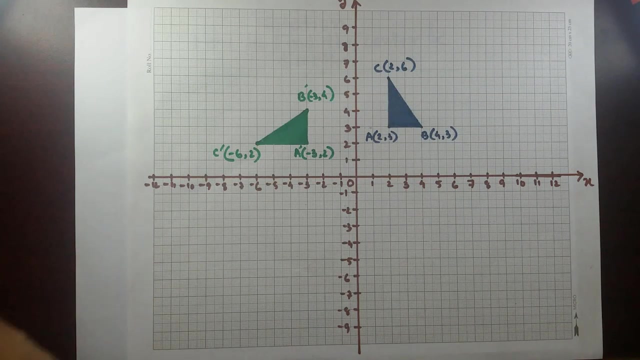 I'm gonna go back again. okay, That's my object and that's my image. okay, So this, using tracing paper. this is another way of doing this, But the easiest way if you cannot, if you cannot find out in trial and improvement method. 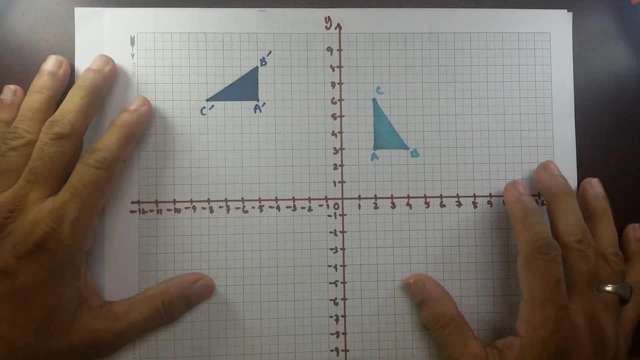 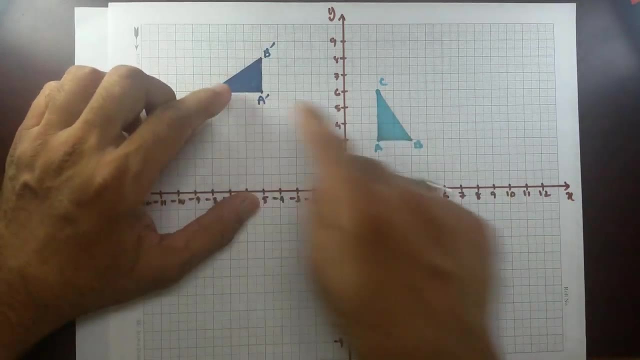 there is a geometrical way to find it out. see this too: If I take this triangle A, B, C, and this is A prime, B prime, C prime, and these two are not rotated through the center, zero, zero. 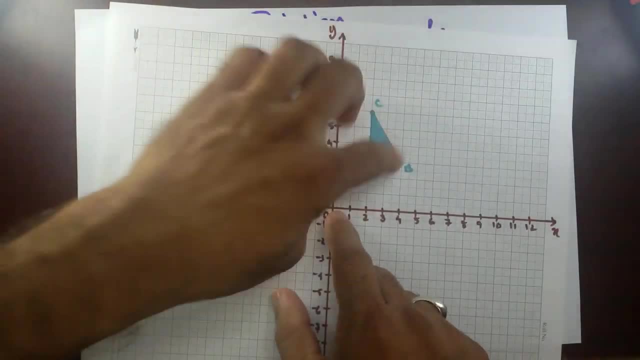 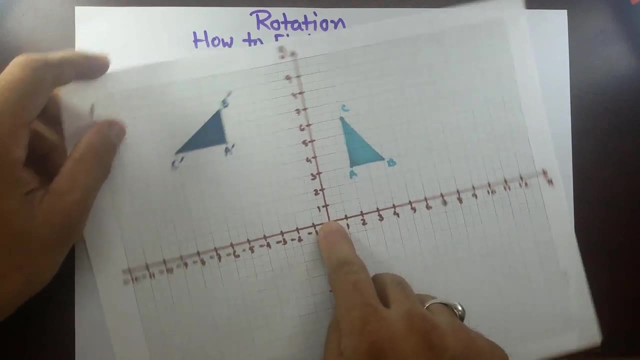 I can see it's 90 degrees somewhere over here. okay, Because it's in the second quadrant. so 90 degree over here, but center is not zero. zero. You can try that if you rotate 90 degree, three units to the left and two units up. 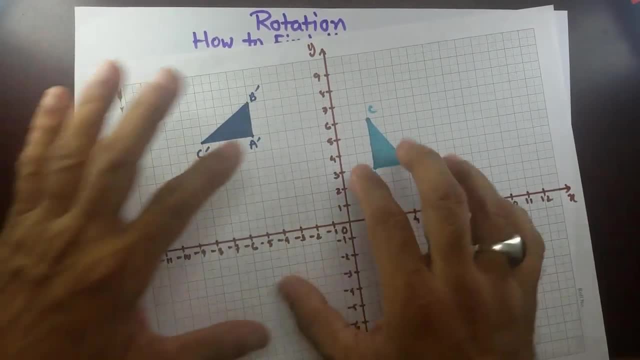 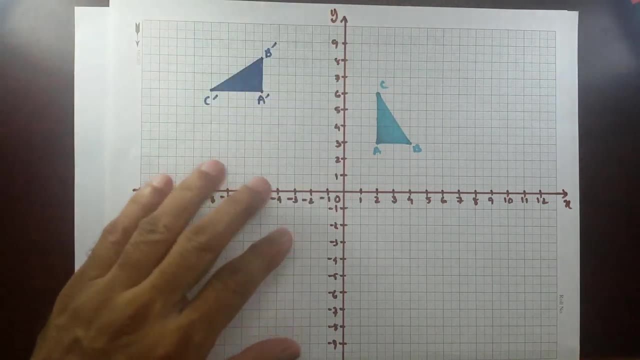 Go back again, three units to the left, two units up. So this is not gonna be working. What can we do? And this is gonna be true for everything. What the first thing you need to do? join any two corresponding points. okay. 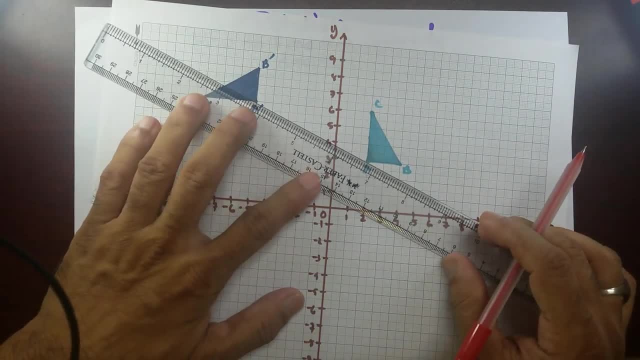 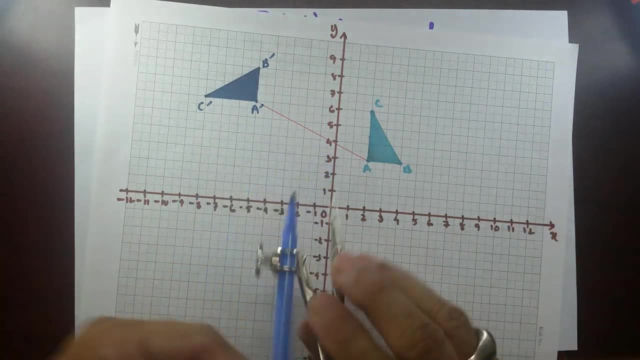 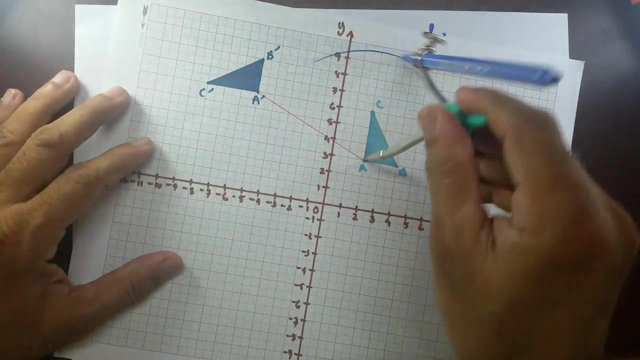 I'm joining AA prime. okay, You can join any two corresponding points. I'm joining AA prime And what I'm gonna do, I'm gonna do the perpendicular bisector. So from here, if I have this arc on the both sides, 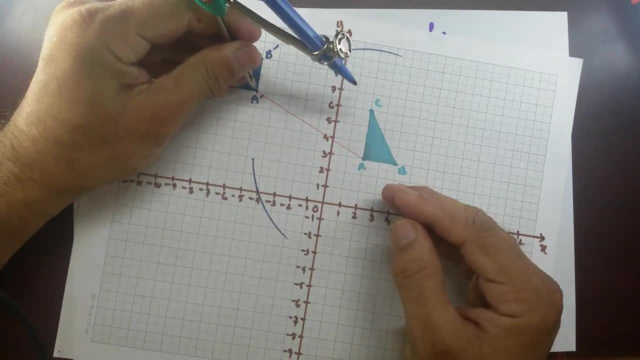 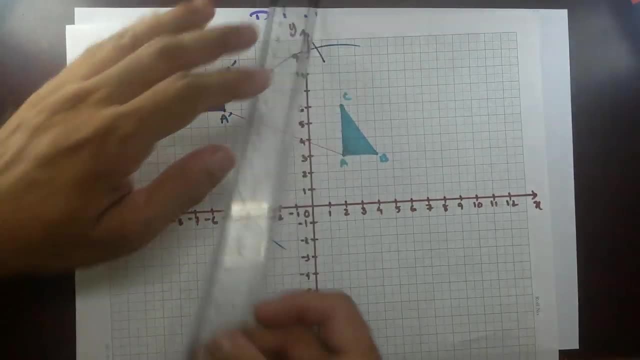 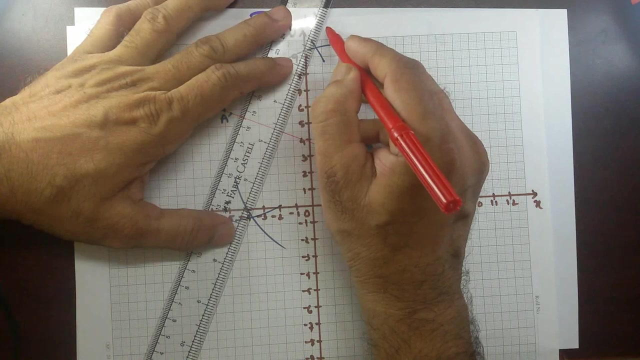 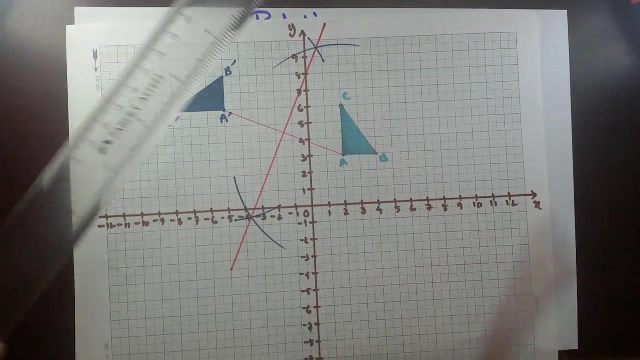 of AA prime and from here, if I join this and I have the palm tree type of thing over here- join this two and when you join you're gonna get a perpendicular bisector of AA prime. okay, I need one more, one more, pair of corresponding points. 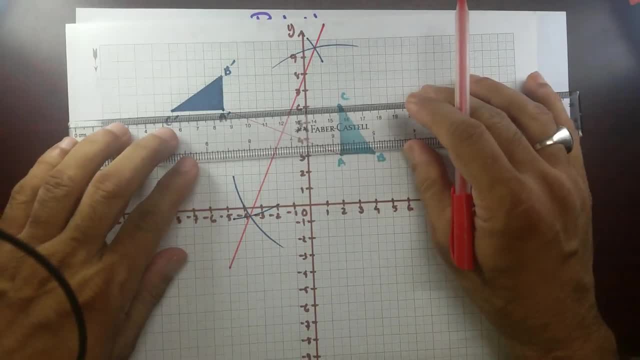 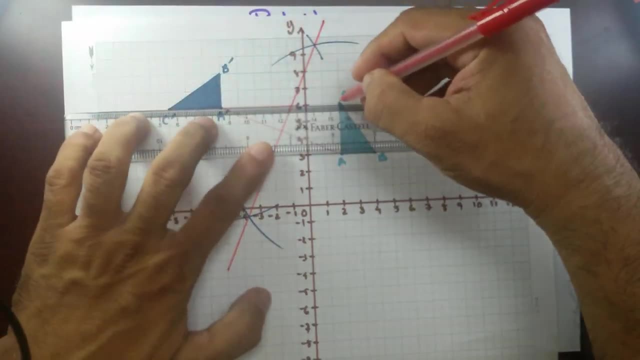 So I can go and I'm gonna draw this point And and that's it. So I'm gonna rely on my point C, prime. Okay, that's probably gonna be the easiest because it's horizontal line. So it doesn't matter. it doesn't matter. 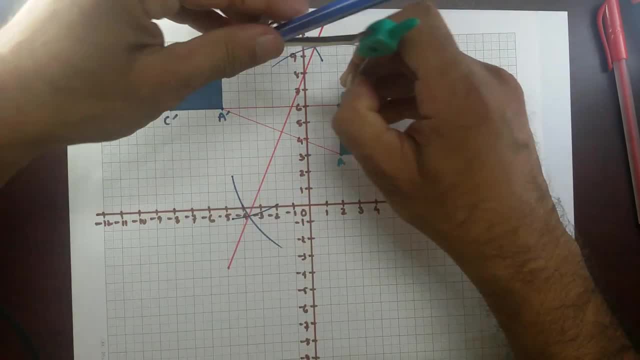 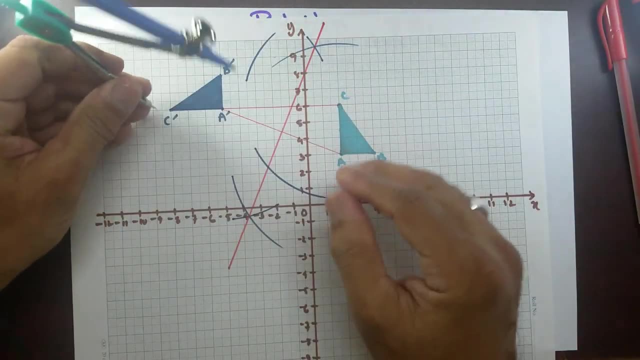 You can take BB prime as well. okay, So that's that. Now draw the perpendicular bisector of CC prime. So this is my point C- And remember to take more than half of this, otherwise it's not gonna be intersecting. 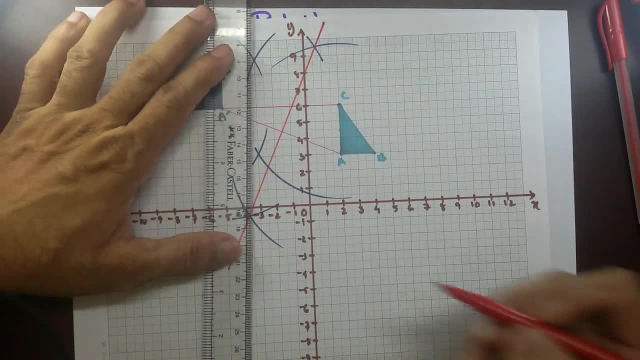 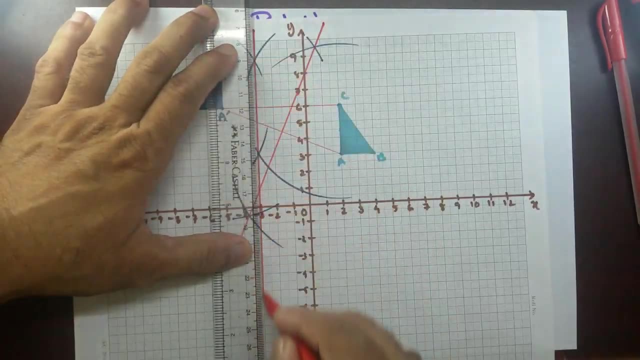 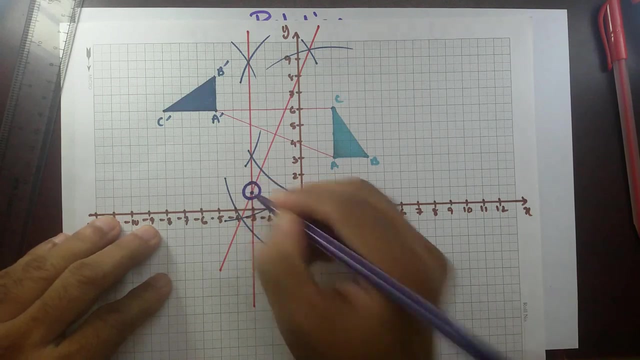 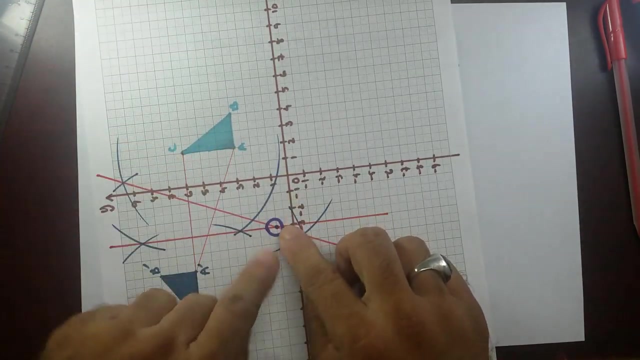 when we join this, when we are joining this, then I'm having these two perpendicular bisector intersect at this point, this point. okay, This might be the center. okay, Let's see if I turn it around this way. so A is gonna be two units this side. 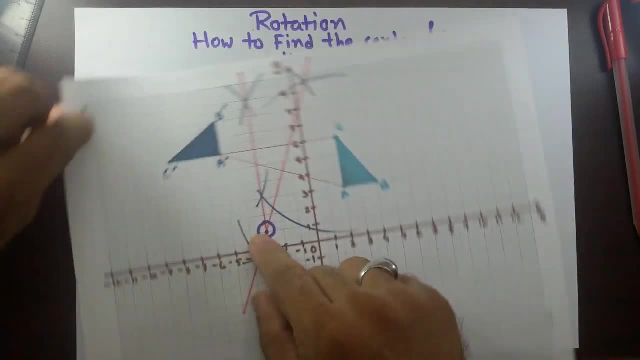 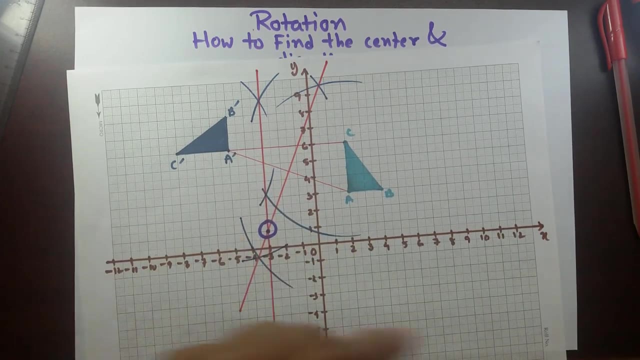 one, two, three, four, five, five units up. so going back again, two units this side: one, two, three, four, five. so this is the center. okay, There is to be sure that, if you're right or not. 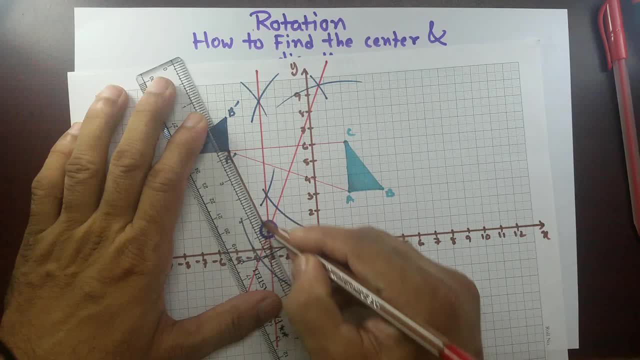 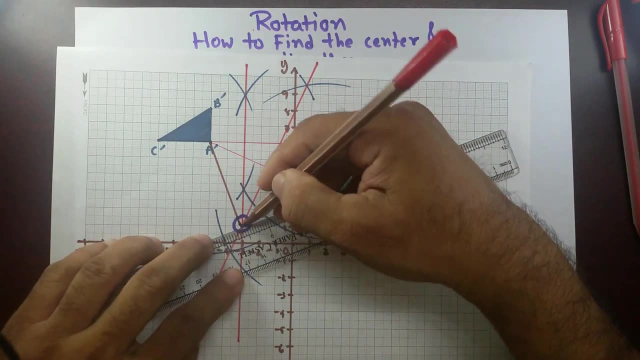 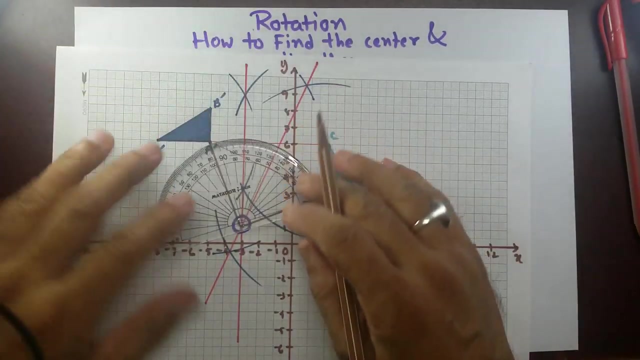 what can you do? You can join this two corresponding points. I join with the center A prime and join from the center A. see that triangle angle you make And take the protector and see if it's 90 degree or not. See it's 90 degree. 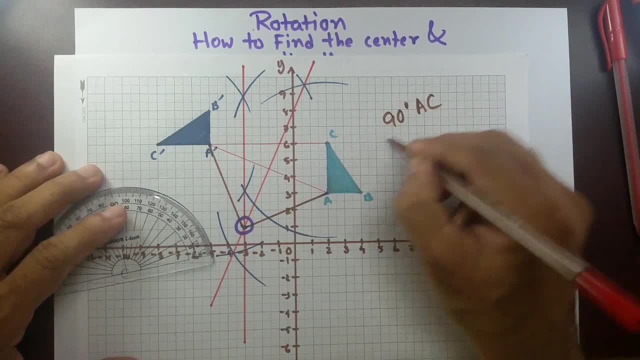 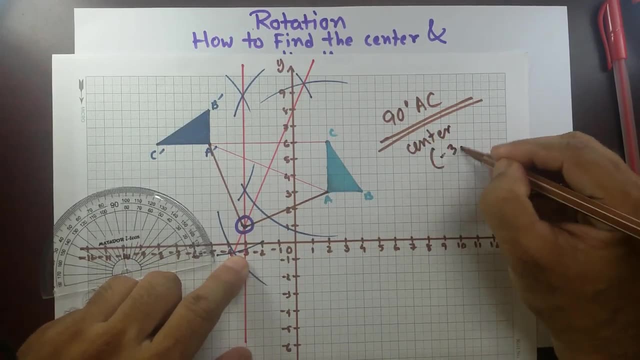 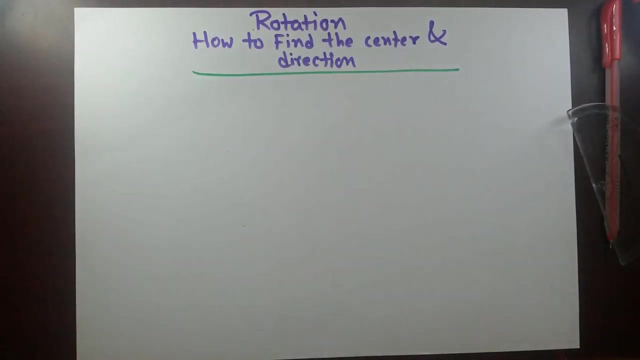 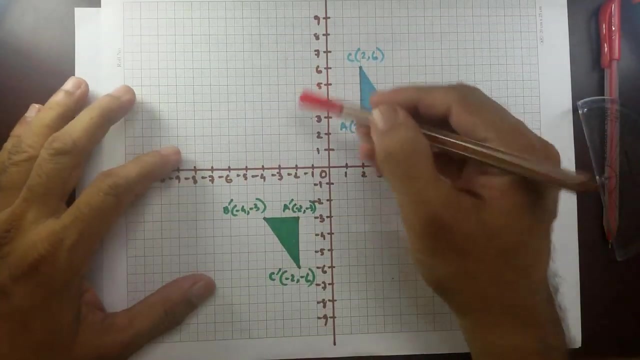 So this rotation is 90 degree, anti-clockwise, okay, And center, center would be minus three, minus three and one. okay, This is how you do that. And the last one left is the 180 degree. 180 degree is in the second quadrant. 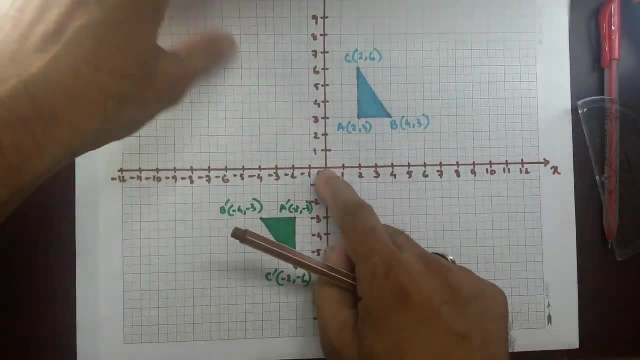 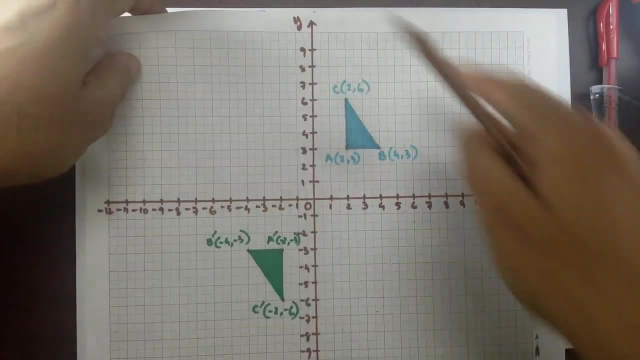 oh yeah, third quadrant, first quadrant, second quadrant, third quadrant, third quadrant. It shows that it's going to be 180 degree rotation. so it doesn't matter if you go anti-clockwise or clockwise. You can try trial and improvement method. 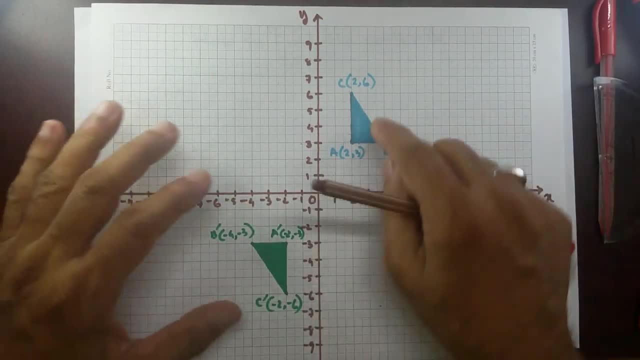 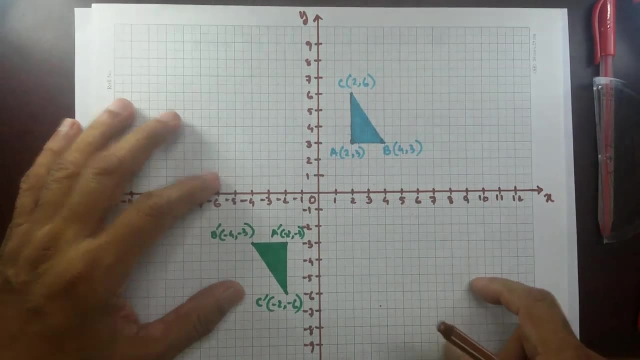 you can try tracing paper, but I don't recommend that You can just join two pair of corresponding points, two sets of corresponding points, and perpendicular bisect them and wherever they intersect, that's gonna be your center of rotation, okay. 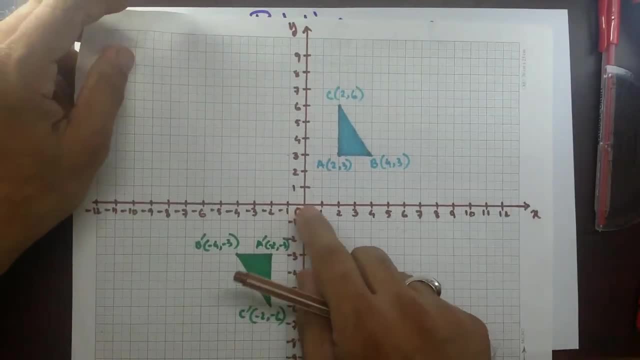 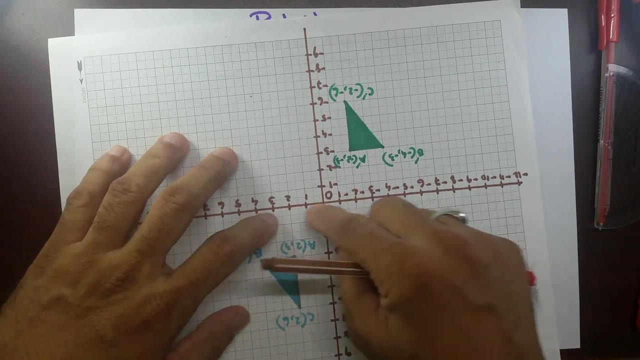 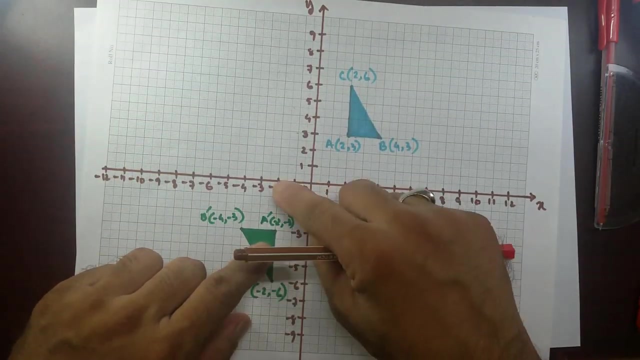 In this case zero, zero. Okay, see that When I go at 180 degree rotation it's negative sides of X: two units this side and three units below. So go back again. See, this image is negative, two sides this way.